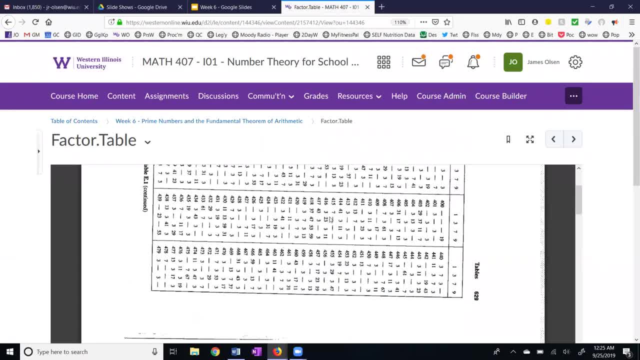 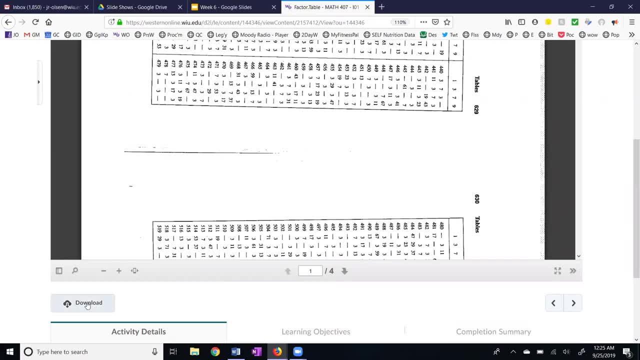 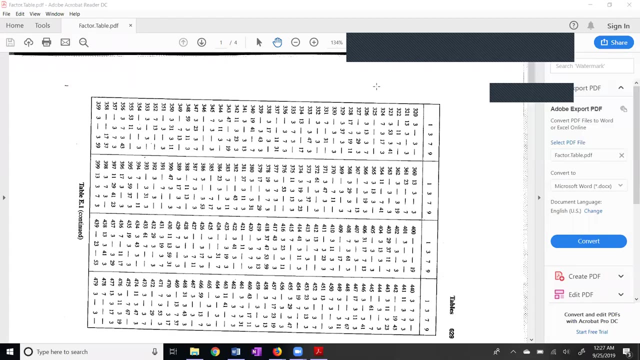 The first thing we're going to need to do here is open this up in something that we can rotate it, So I'm going to download this. Okay, I have the file opened up in the Adobe Reader here, And here in the View menu is Rotate View. 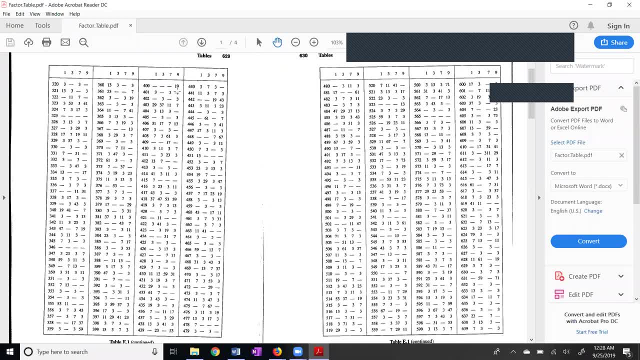 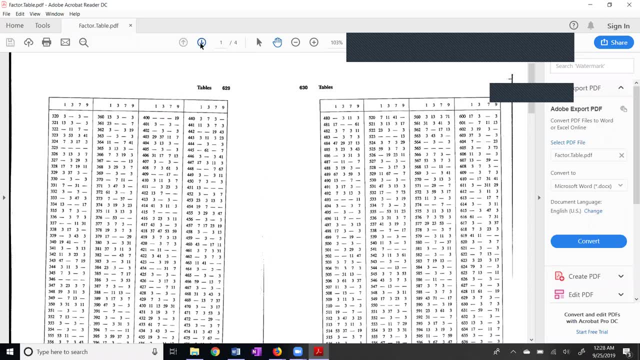 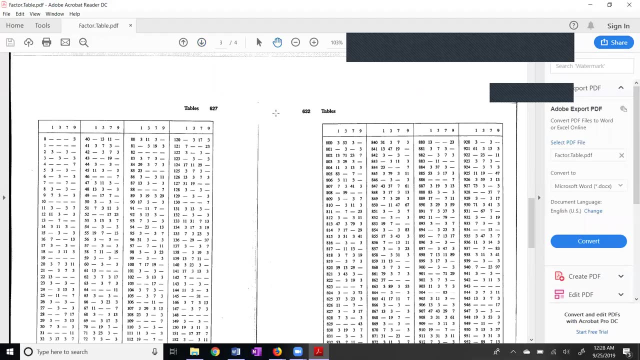 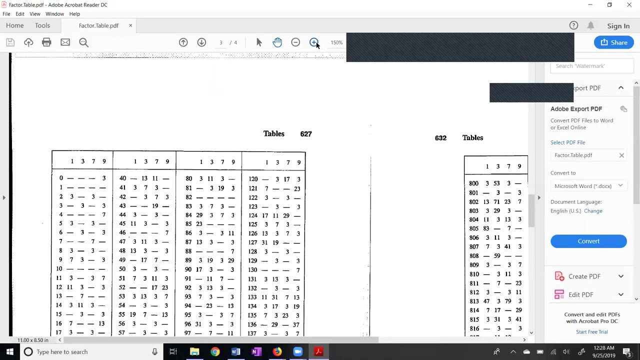 So here is a couple of the pages: page 629 and 630.. This needs to be rotated. Okay, right, here is actually the beginning of the table. Okay, Okay, Let's take a look at the beginning of the table and see how to read this. 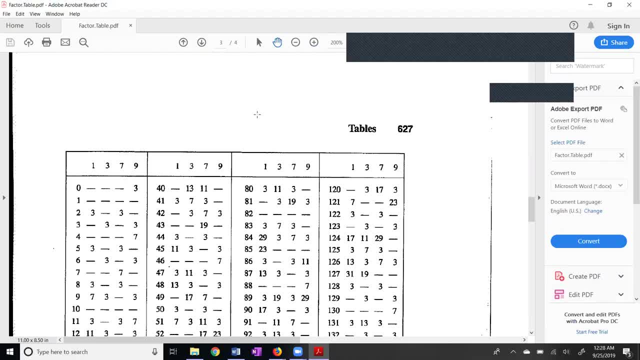 First of all, first principle is: this table only has odd numbers in it Because an even number is going to be divisible by two and you can always take out factors of two until you get an odd number. What is being shown in the body of the table is the smallest prime number that divides into the number. 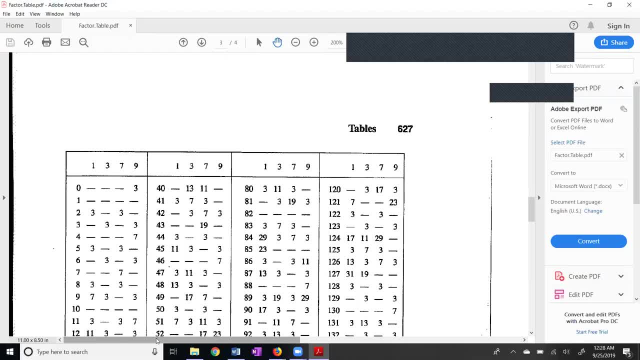 So let's take a look Here. let's take the number 63,, for example. where's the number 63?? I find six right here and I use the column three and that makes a two digit number. 63 and three is the smallest prime number. 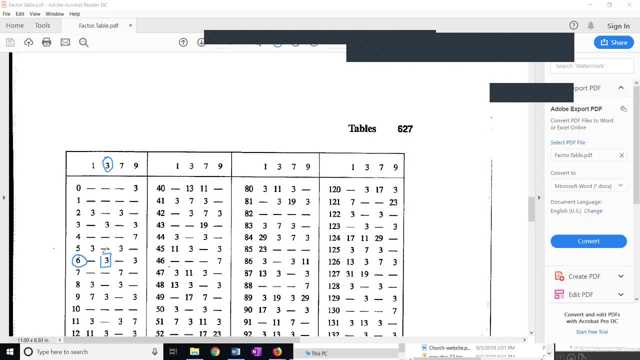 That divides into 63. So what you might do is take 63 divided by three and get 21.. Then find the smallest prime number that goes into 21.. Well, 21,. let me change my color here. 21 is going to be right here. 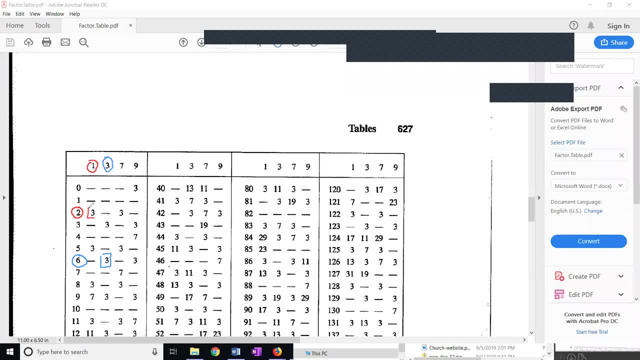 The smallest prime number that goes into 21 is also three. So I would take 21 divided by three and get seven. Now the number 7 would be- and let me get a third color- the number 7 would be right here- 0, 7, kind of trivial. 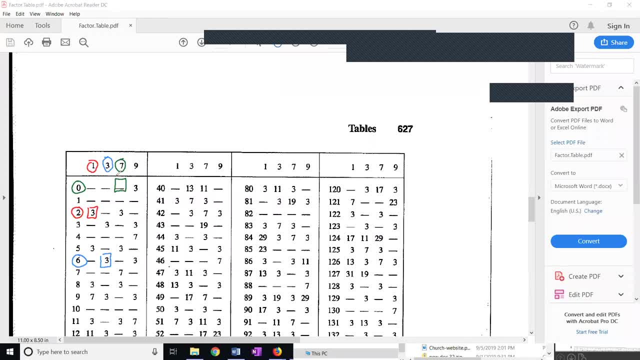 When you see a dash, that means you have a prime number. So let's take, for example, 89.. Let's look at this table and see if 89 is a prime number or not. 89, here's 8,, here's 9, and we see a blank. 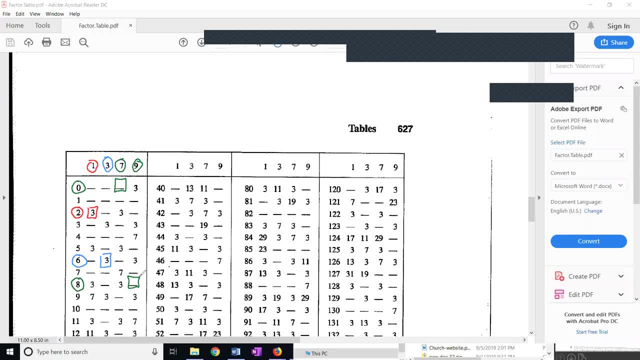 The blank means it's a prime number. Okay, so those are the small numbers. Now let's see if 861, 861 is a prime number. I find the first digits here, 861. here, And we see, I find that 861 is not prime, it's divisible by 3.. 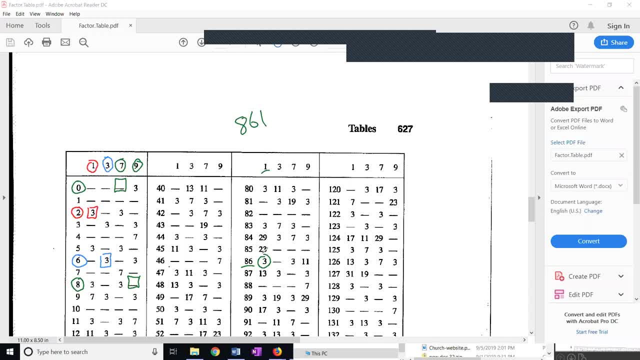 However, 863 is prime 3 divides 861.. By the way, we could use a divisibility test on that, But the nice thing about this table is it's useful for things I can't do the divisibility test on All right, so there's some simple examples. 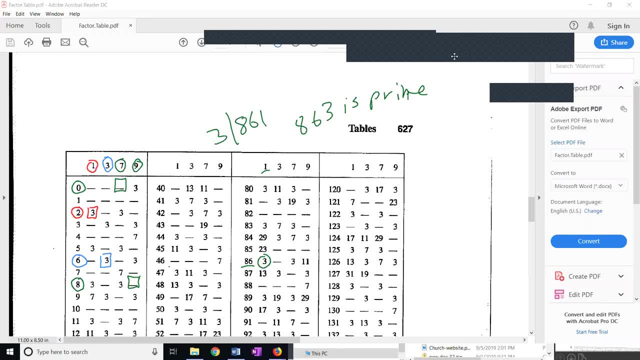 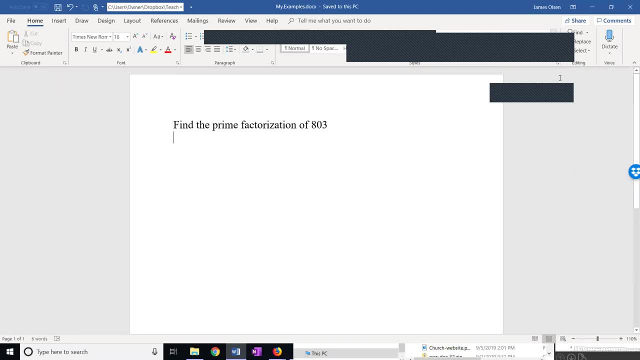 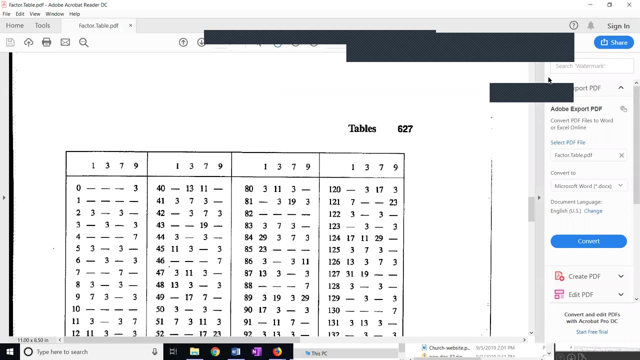 Now let's do something significant. I'd like to find the prime factorization of 803.. So we come over to our table and find 803.. By the way, this is much easier to use the print table than the computer, But since this is an online, 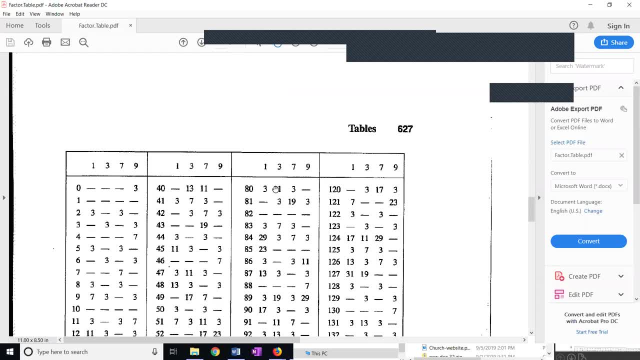 This is an online video. I have to do it. 803 is right here. 803 is divisible by 11.. So I'm going to take 803 divided by 11 on a calculator. 803 divided by 11 is 73.. 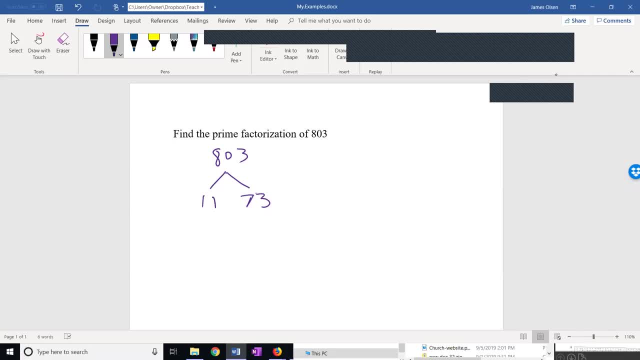 And if I look in the table I see that 73 is also prime, So we have 803.. And if I look in the table I see that 73 is also prime, So we have 803 divided by 11 on a calculator. 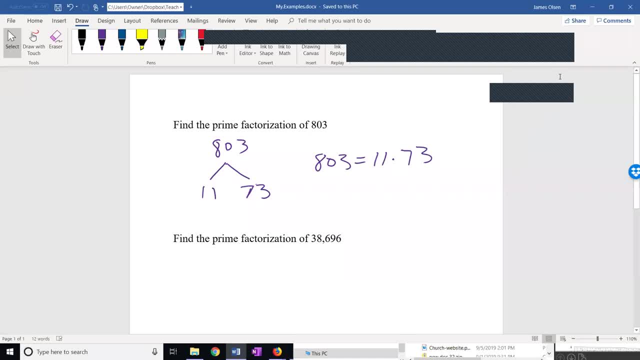 So I then subtract 303.. So according to that equation, we can see that 303 is equal to 11, times 73.. Now let's do another one. Now we'd like to find the prime factorization of 38,696.. 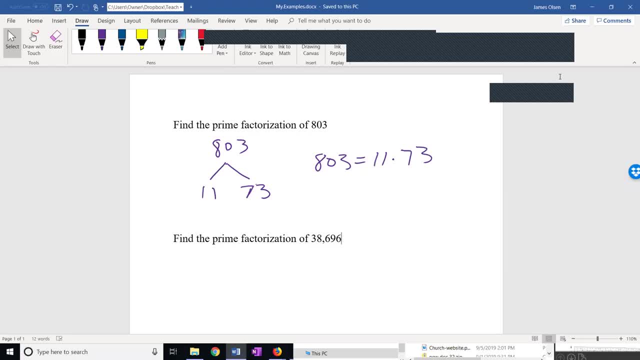 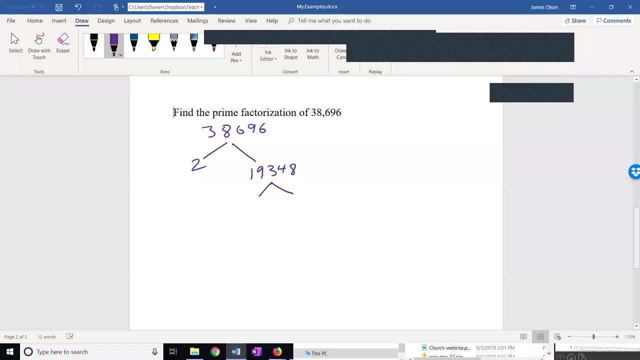 And this is bigger than that. but the good news is this is an even number, So you should take out the even numbers by hand first. So go ahead and start the factor tree, Continue taking out 2 as long as you have an even number. 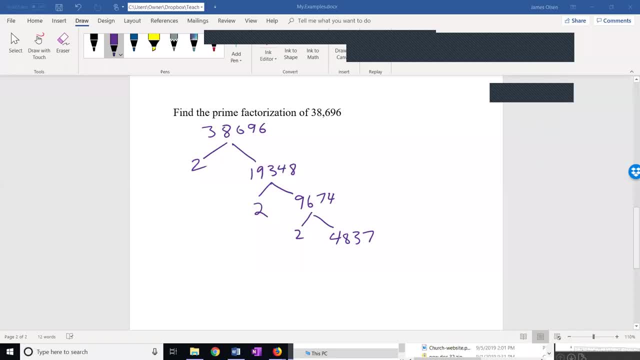 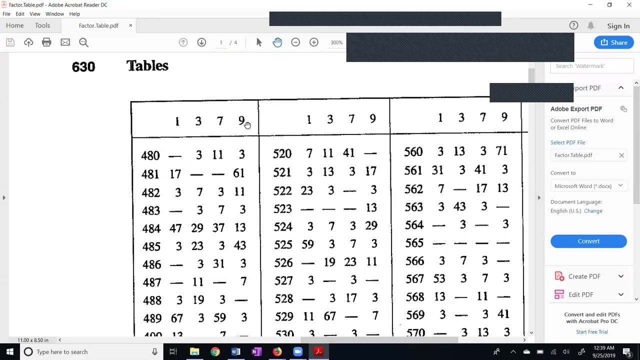 So so far I have 2 times, 2 times 4,837.. Now we need to look up 4,837 in our factor table. 4,837,. here are the first three digits and the final digit is at the top. 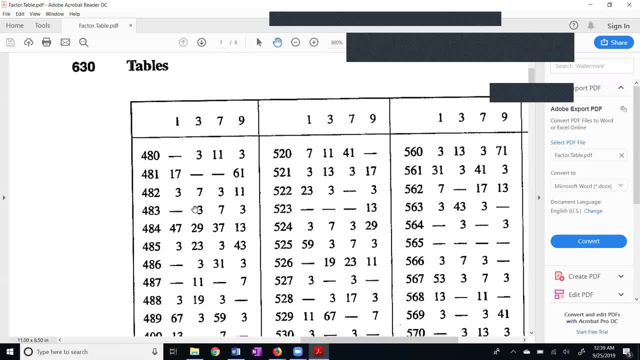 4,837 is not a prime number. 4,837 is a prime number, 4,837 is a prime number, 4,831 is a prime number, but 4,837 is divisible by 7. So I'm going to need to divide that by 7 on a calculator. 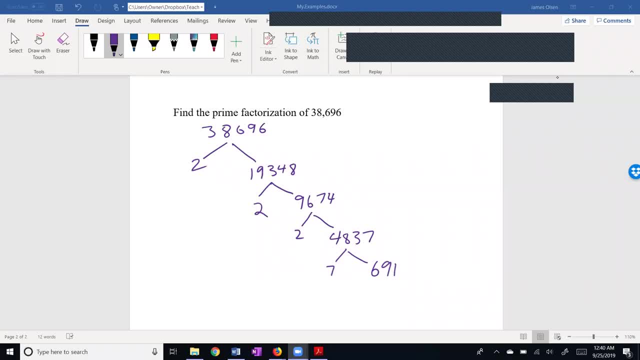 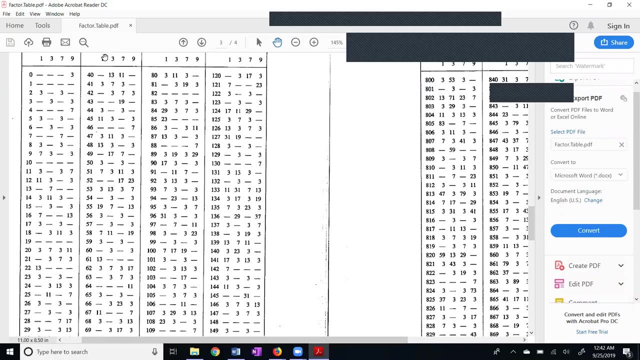 I get 691.. Now I need to find out if 691 is a prime or not. so I'm going to go back to my table. 691,, here's 69, and here's the 1 column, and I do see the dash right here. so 691 is a prime number. 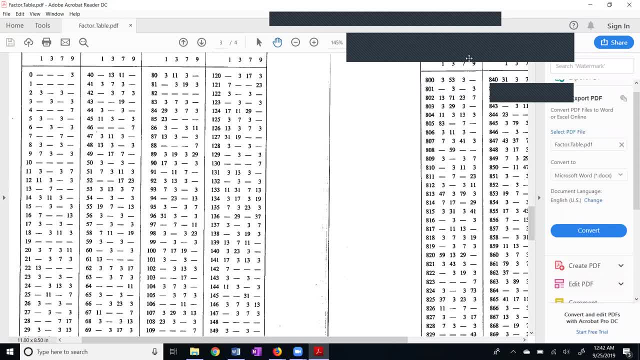 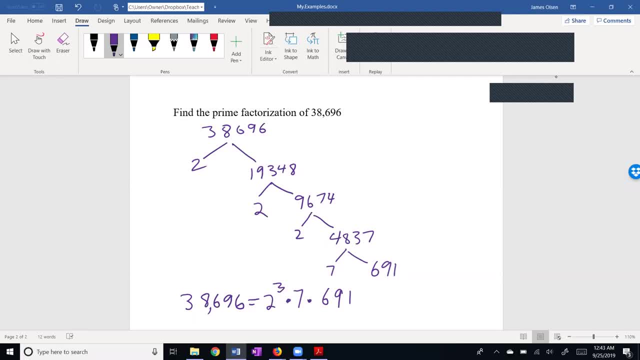 So now I can write my prime factorization. My prime factorization: 38,630.. 96 is equal to 2 cubed times 7, times 691.. Our next topic is the sieve of Eratosthenes. 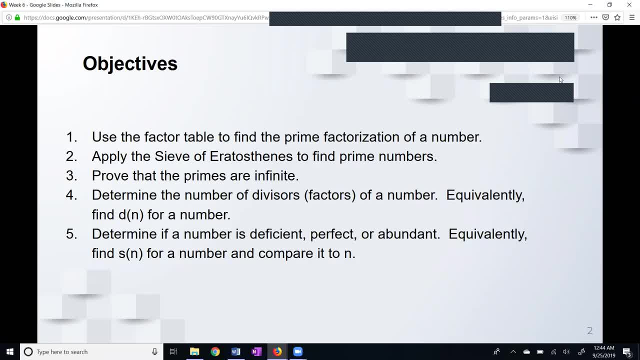 This is a very interesting thing historically because this was made up by a Greek mathematician. I believe he was in Allegheny, I believe he was in Alexandria in Egypt. So there are some nice websites for the sieve of Eratosthenes and this is also explained in our book. 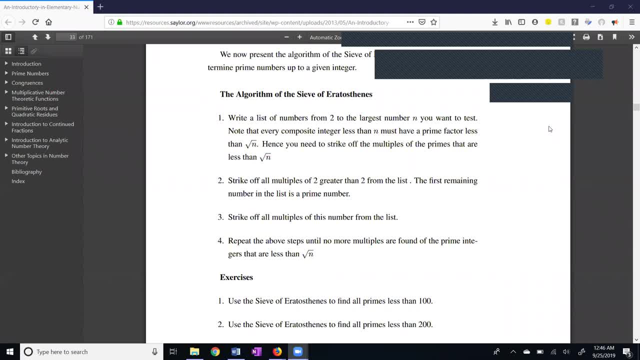 So here's the algorithm of the sieve of Eratosthenes. It's easiest to understand if we look at an example. The first thing we're going to do is make a list. The first thing we're going to do is make a list of the numbers, either starting at 1 or 2.. 1 is not a prime number. To be a prime number it must be a positive number and it must have exactly two factors. 1 has only one factor, So 1 is not prime. 1 is not composite. The first prime number is 2.. 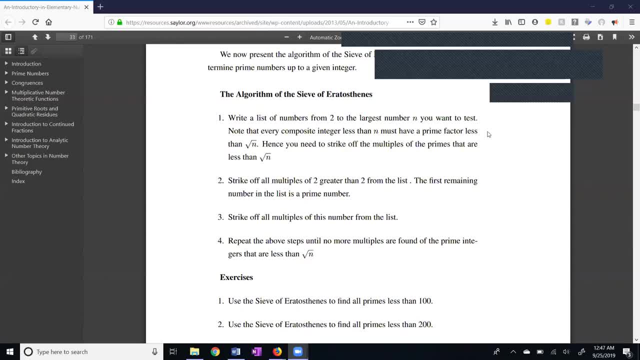 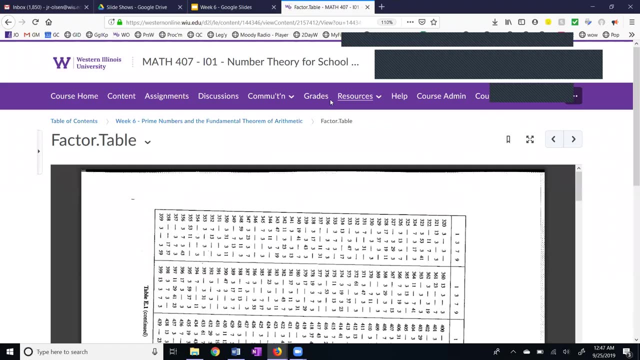 The good news is That we only need to check up through the square root of n. So let me show you an app where we can do this, And this is in our area of resources. So if we come to our website and we come to the links, 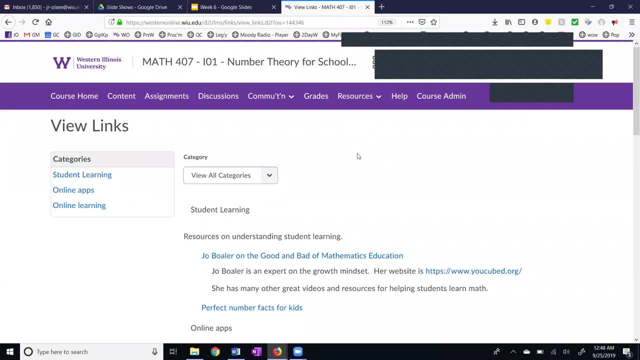 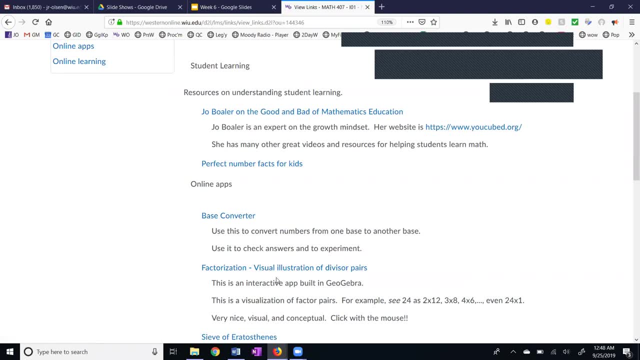 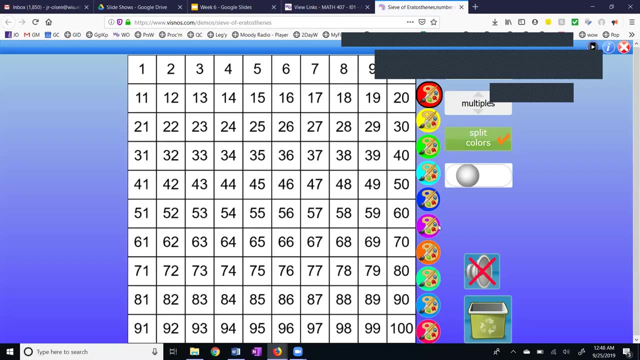 Here I am at the links Which is underneath our resources, And right down here is the visual illustration of the sieve of Eratosthenes. It's what we want tonight, And here it is Now. the first thing I would do is I would speed this up. 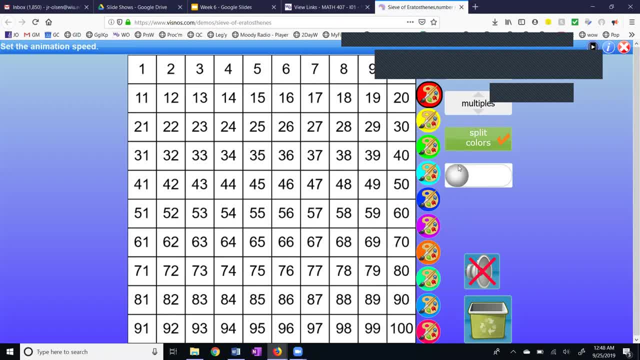 This is the speed here, And what you're going to do is hit the first prime number, which is 2.. And you're going to hit the first prime number, which is 2.. And you're going to hit the first prime number, which is 2.. 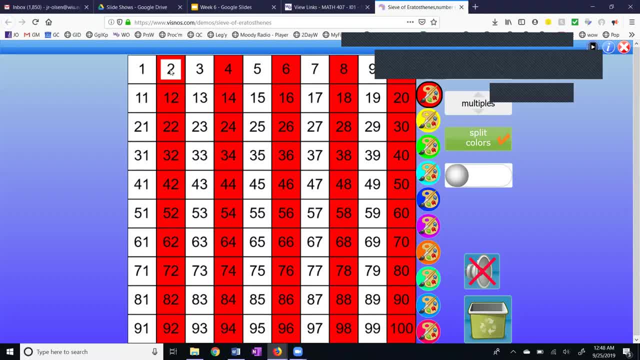 And it's going to color in all the multiples of 2.. This one that has the box around it is a prime number. The ones that are shaded in are no longer candidates for prime numbers And you come with a different color And you come to the next number that is not shaded in. 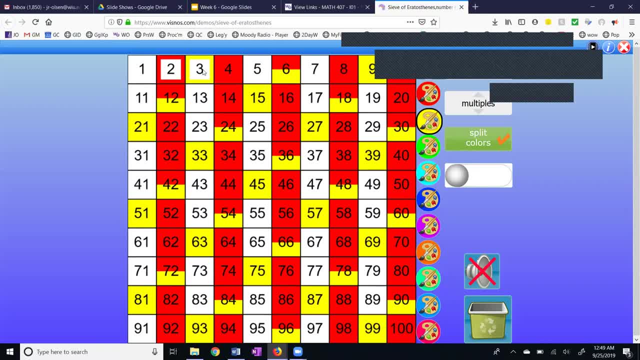 And shade in or cross out all the multiples of 3.. Maybe I'll slow it down a little bit. See if I can slow it down for 5.. Then you do 5. All the multiples of 5. And you color these in. 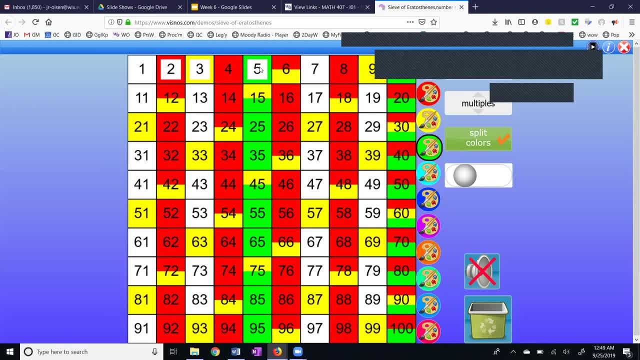 Now, of course, some of them have already been colored in already. Then you color in all the multiples of 7. And this eliminates those. Now we are done. If we're only interested in the primes up to 100, the square root of 100 is 10.. 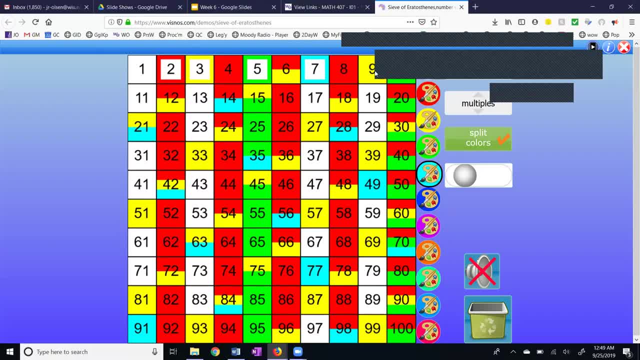 So I don't really need to worry about 10 or 9 or 8, because those are not prime numbers. The largest prime number less than the square root of 100 is 7.. So here is a listing of all my prime numbers. 2,, 3,, 5,, 7,, 11,, 13,, 17,, 19, and so on. Up in the 90s there's only one prime number, It's 97.. In the 80s, there are two prime numbers. 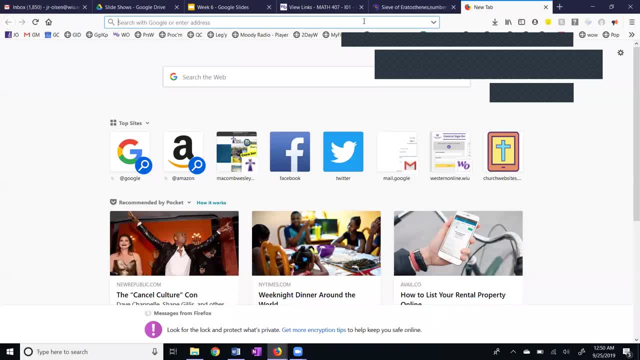 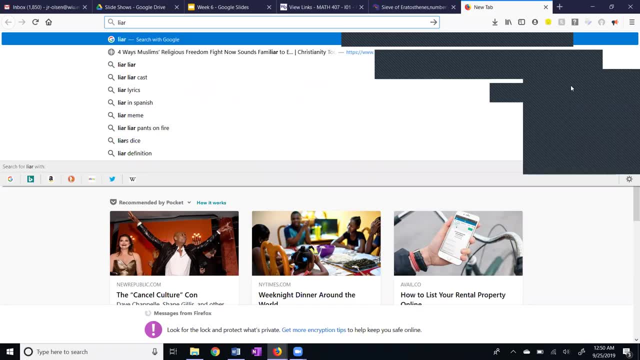 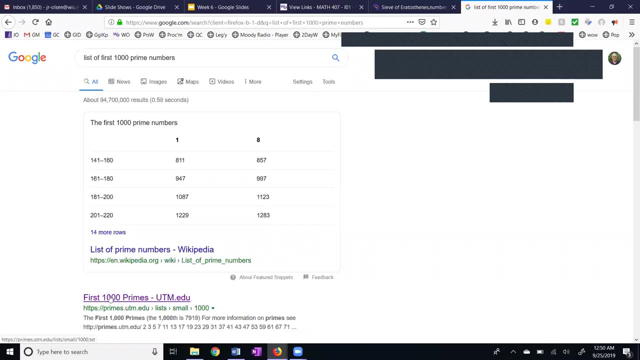 Now what you might do is is Google for list. I can't type list of the first 1,000 prime numbers, for example, and over here is a good website and this is the first 1,000 prime numbers. 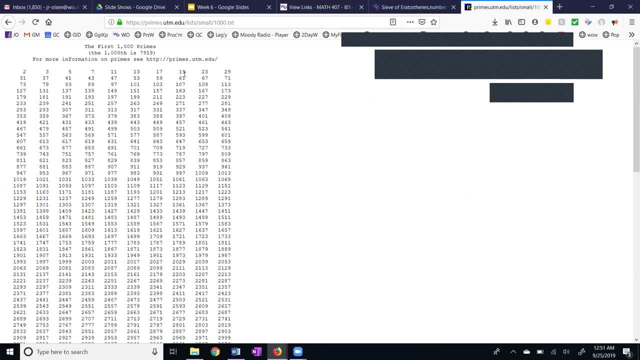 two, three, five, seven, 11,, 13,, 17,, 19,. and we see here, in the 80s there are two numbers and in the 90s there's only one number. that's a prime number. 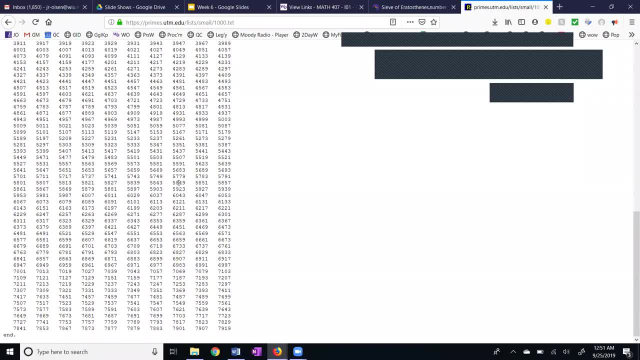 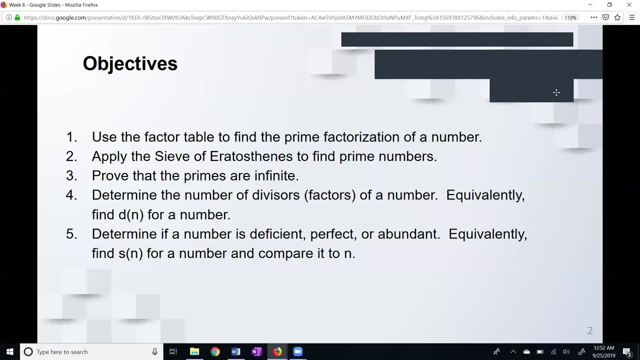 The 1,000th prime number happens to be 7,919, and you might verify that on the factor chart. The third thing I'd like to do is prove that the primes are infinite. The primes do get thinner and thinner the higher you get. however, they do go on forever. 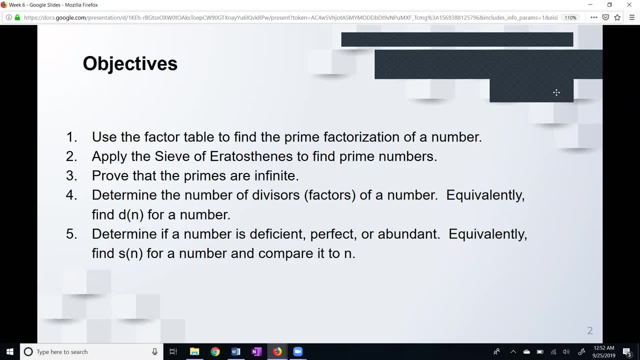 and of course, this was of great interest early on in mathematics. and the Greeks also proved that the primes are infinite. My proof is going to start out similar to the one by our author, but my proof is going to end up a little bit different. well, the end will be the same. 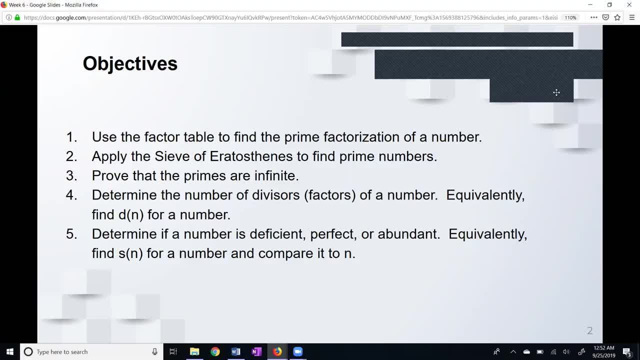 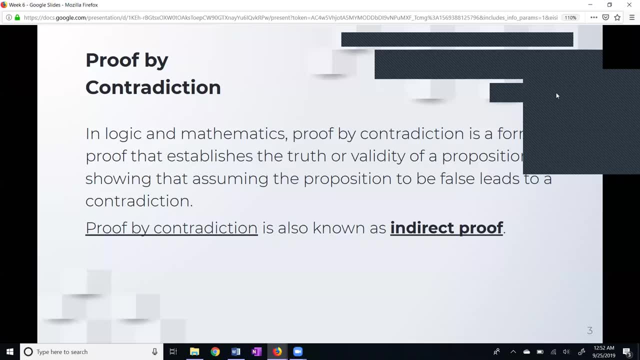 but the second half of the proof will be a little bit different. It's going to be a proof by contradiction. What is a proof by contradiction In logic and mathematics? a proof by contradiction is a form of proof that establishes the truth, the truth or validity of a proposition by showing. 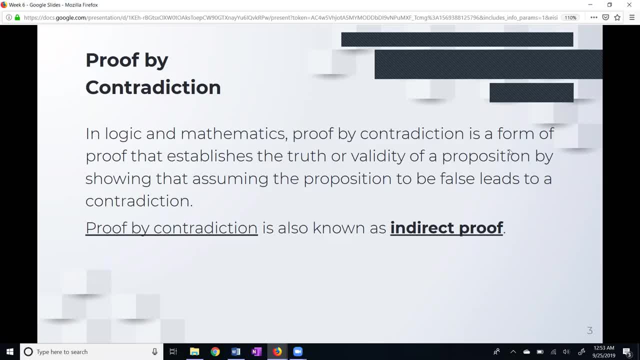 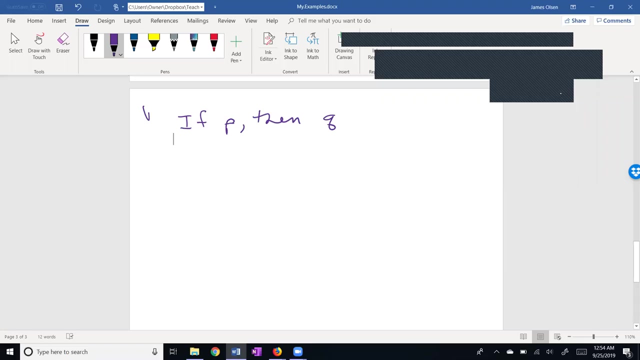 that assuming the proposition is false leads to a contradiction. A proof by contradiction is also known as an indirect proof. So let me see if I can explain this a little bit. Let's say we're trying to prove the statement: if P, then Q. 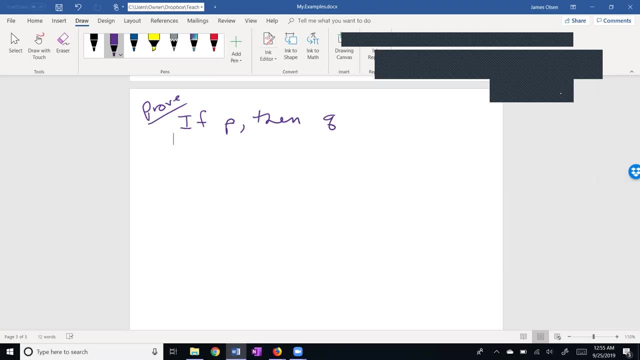 P is our given information, and Q is our given information. Q is our conclusion. Now, Q is either a true statement or a false statement. There's only two possibilities. So what we do here is: this is a proof. so we should start out by saying that this is a proof. 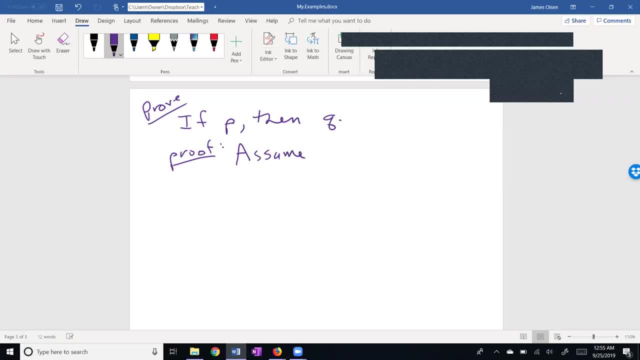 We're going to assume, and sometimes for emphasis, we write down for the purposes of contradiction. for the purposes of contradiction, This signals your reader that this is going to be an indirect proof. You start out with, not Q, The negation of the Q statement. 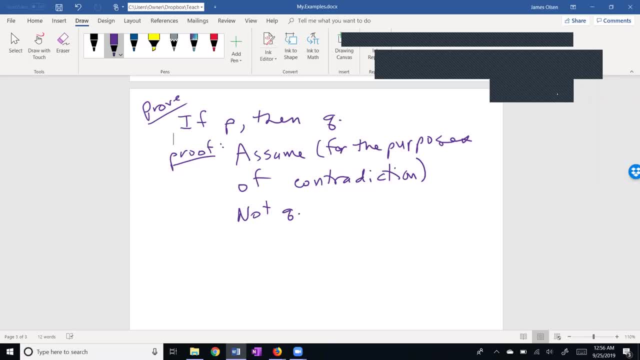 And one thing about individual proofs is that it comes from the statement itself, And so why is it a proof? Why is it not? Why is it not? Why is it a proof? And one thing about an indirect proof is it kind of gives you a little bit of extra information. 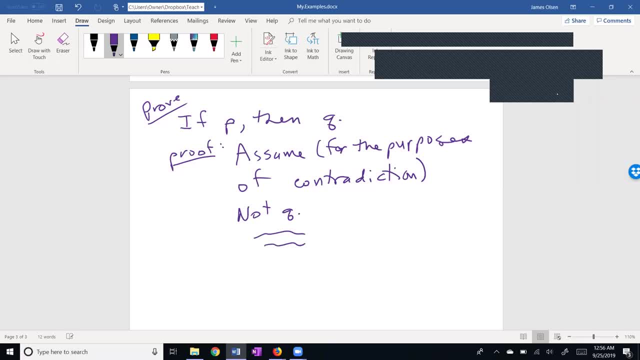 And then you start logically making deductions until you get to a contradiction. It might be, for example- and I'm just making up this example- that you get to something like X equals 19.. And then later on in the proof you get to X equals 3.. 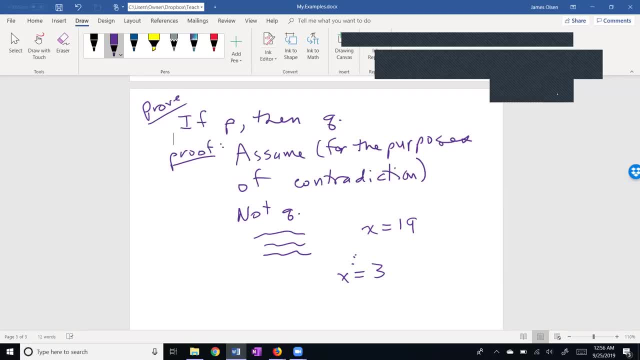 That's a contradiction. You cannot have X equals 19 and X equals 3 at the same time, So the ending of a proof by contradiction always ends the same way. Once you arrive at your contradiction, you state: this is a contradiction. Therefore, our assumption is false. 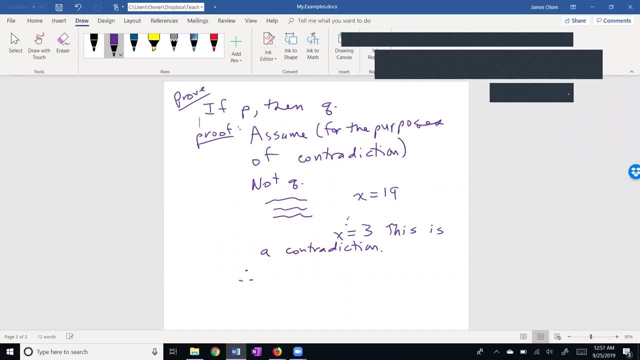 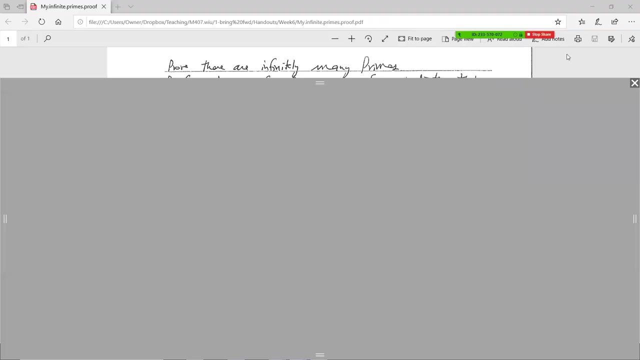 Therefore, three dots. Our assumption is false. Our assumption was right up here, Not Q. Therefore Q is true. Now let's see this in operation. Okay, Take down the following proof in your notes. Pause the video as needed. 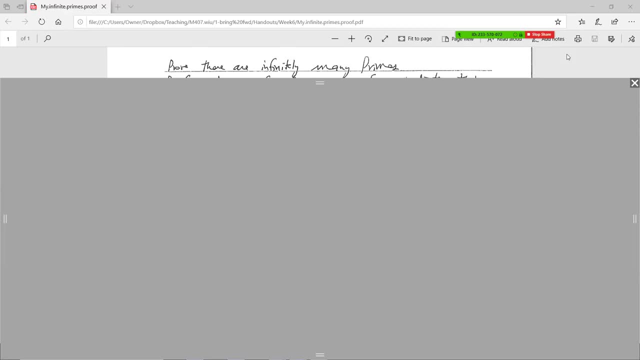 We want to prove there are infinitely many primes. Now there's two possibilities: Either there are infinitely many primes or there are not infinitely many primes, which means there's a finite number of primes. So here's my proof. I'm going to assume, for the purposes of contradiction, that the primes are finite. 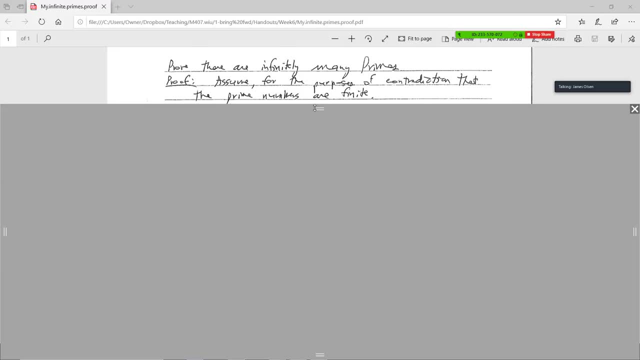 The opposite of being infinite is finite. So I am assuming there are infinite primes. So I am assuming there are infinite primes. assuming, for the purposes of contradiction, that the primes are finite. Well, what does that mean? That means they come to an end. Here's a list of the primes: P1,, P2,, P3, P4, all the way up through. 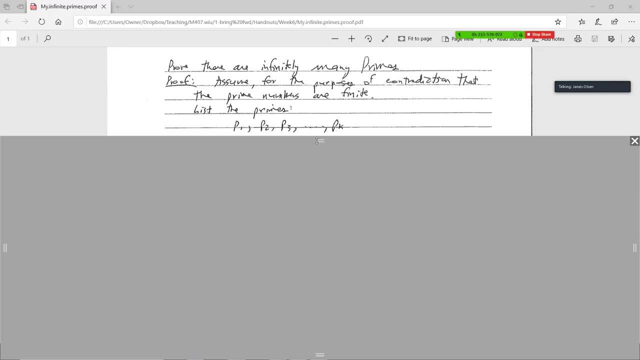 PK. I don't know how many primes there are, but I do know they come to an end. Maybe there's 33,000 or something like that. It is going to terminate at some point. Now what we're going to do is take this finite list. This is not an infinite list. It is a 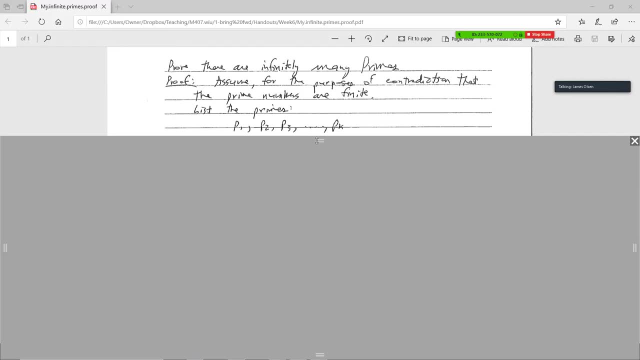 finite list. We're going to take this and we're going to form a big new super duper number and I'm going to call it P star, P star, P star is equal to the product of all of our primes: P1 times P2, times P3, up through PK. and then I'm going to add 1 to it. 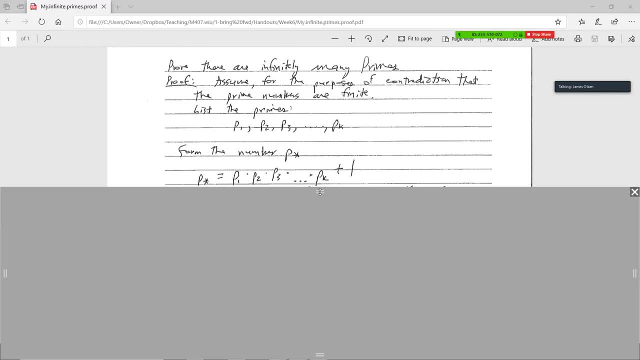 This is going to make a super duper big number. Now you might think about what this P star is. On the one hand, it's bigger than any of our prime numbers, so therefore it's composite. On the other hand, it's composite On the other hand. it's composite On the other hand. 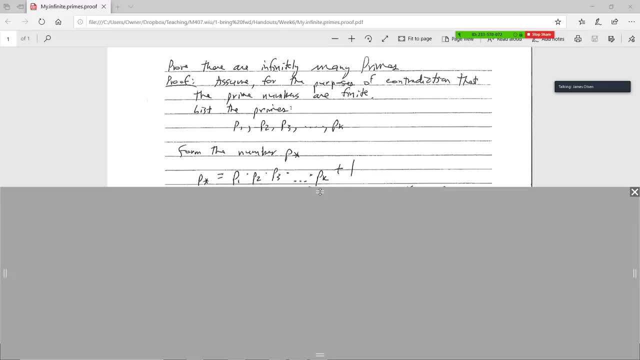 it's not divisible by any of the prime numbers, so we're going to have a contradiction. So let's see how the rest of the proof goes. P star is larger than all the primes. Therefore it is composite. Now, if we think about the division algorithm, if I would divide by P1,, 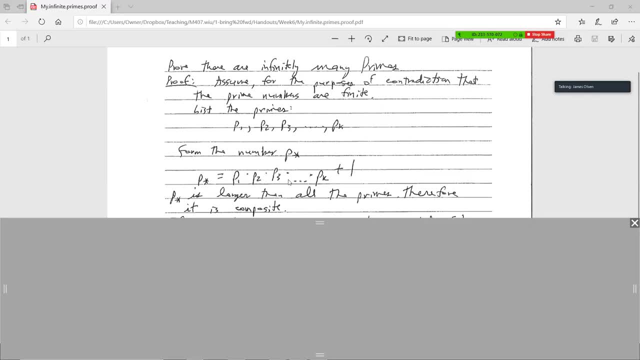 if P1 was my divisor, here would be my quotient: P2 times P3 up through PK, and here would be my remainder. If we divide P star by P1, we get a remainder of 1.. P1 is not a divisor of P star. 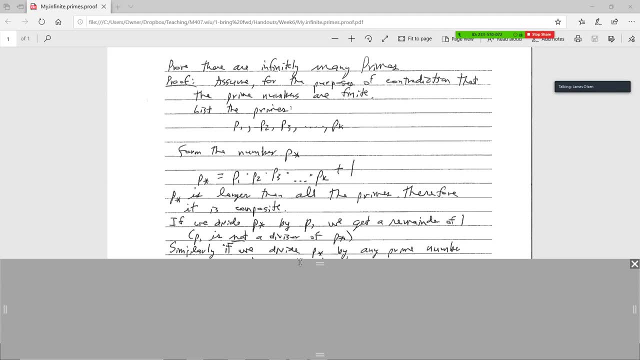 Similarly, if we divide P star by any prime number, the remainder will be 1.. Therefore, P star is not divisible by any prime number. Therefore, P star is prime. Maybe you notice our contradiction. Up here I have P star being composite and here we have 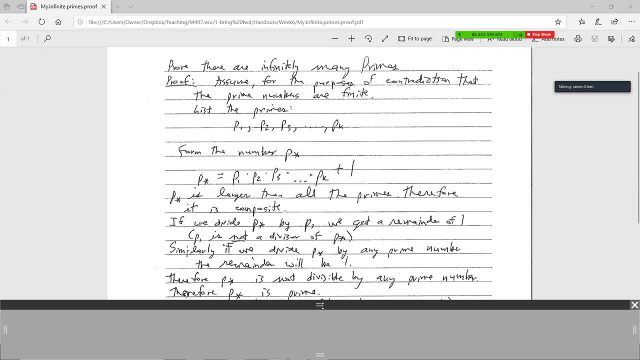 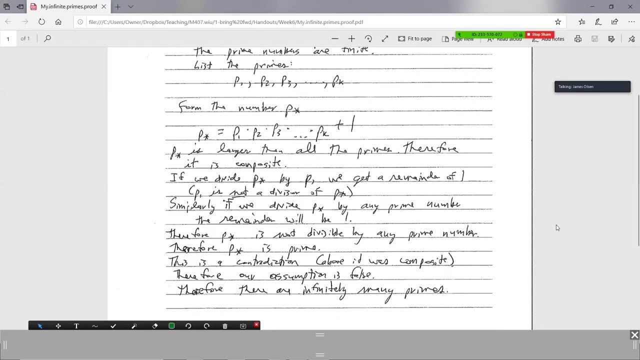 P star being prime, You can't be prime and composite at the same time. This is a contradiction. Above it was composite. Therefore, our assumption is false. Therefore, there are infinitely many primes. This is the end of our proof. This is what we were trying to prove. 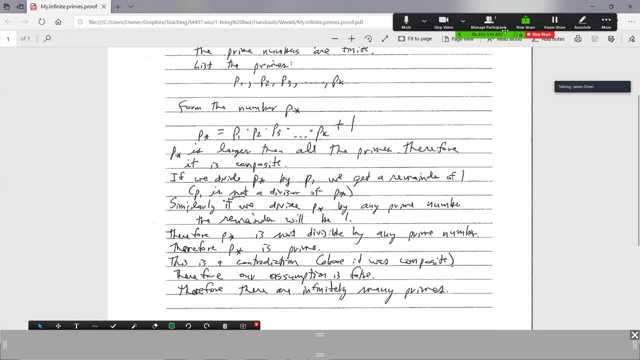 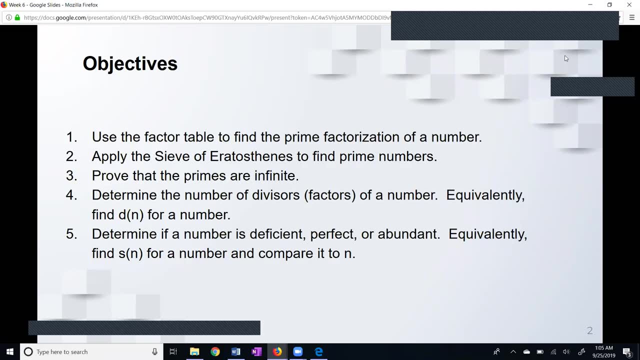 This is the mic drop. Have a cup of coffee. The next thing I'd like to do is show you how to determine the number of divisors or numbers of factors of a number, And, of course, we're going to be using the prime factorization. 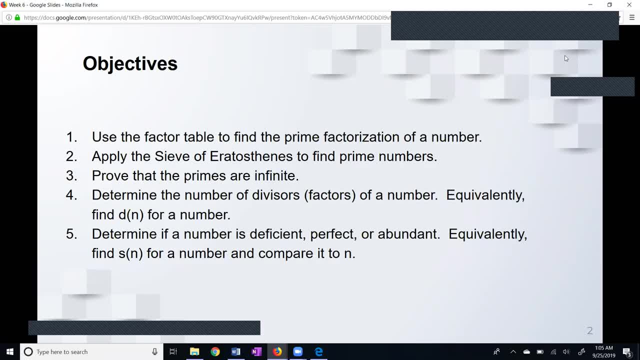 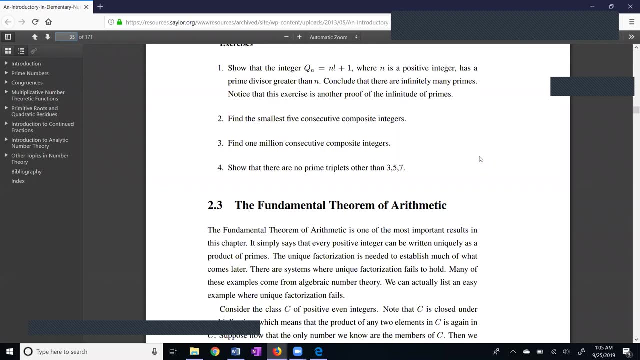 I would be remiss if I did not state the fundamental theorem of arithmetic. So let's find this in our book. The fundamental theorem of arithmetic is one of the most important results in mathematics. They wouldn't call it the fundamental theorem if it wasn't important. 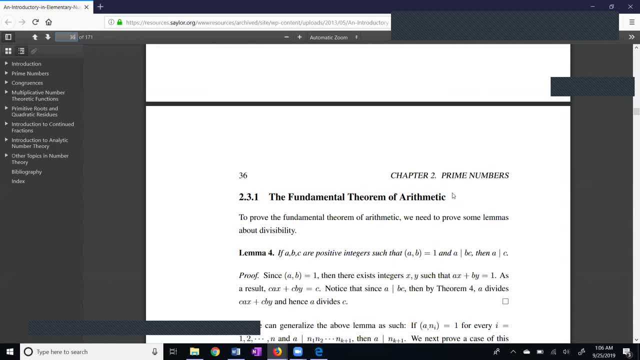 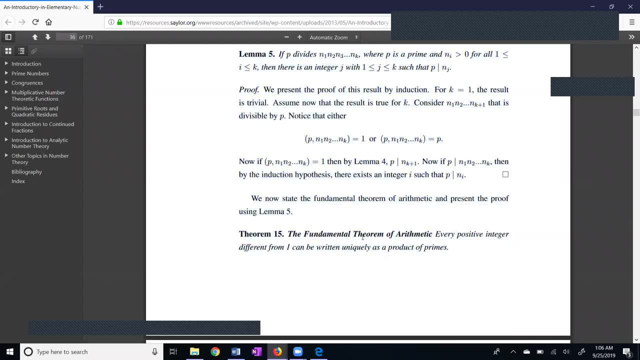 Primes are the building blocks for all numbers. Here is the statement of the fundamental theorem of arithmetic: Every positive integer different from one can be written uniquely as a product of primes. The key word here is uniquely. It means one and only one. So if five different students do the 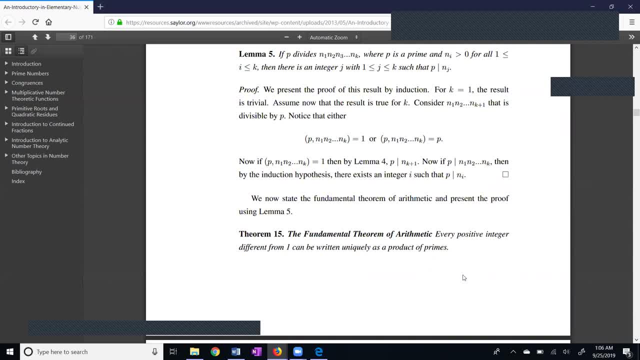 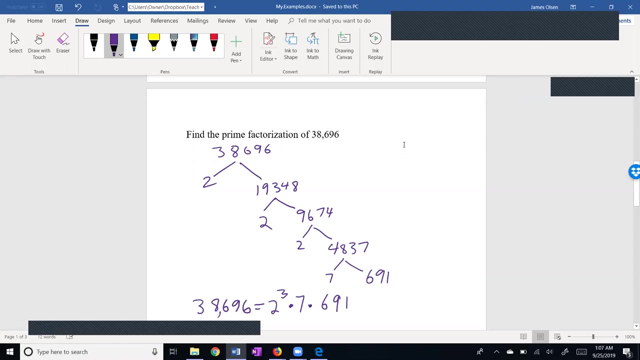 prime factorization of some number make up a number like 484,. each student does the prime factorization. they will all get the same product of primes. So let's take a look at this big number, the 38,696, which we have the prime factorization for. 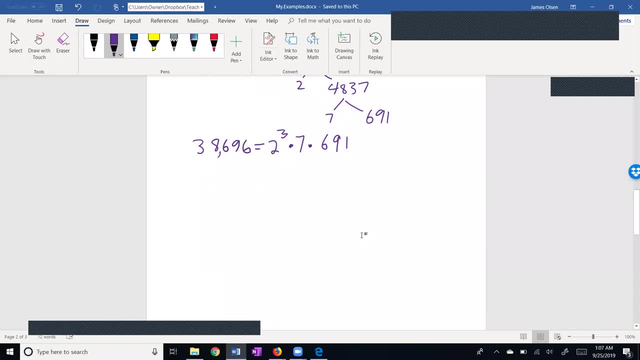 And take a look at the number of factors And I'm going to kind of show you conceptually how to do this and then I'm going to show you how to do it. So let's take a look at this big number, the 38,696,. which we have the prime factorization of some number. so let's take a look at this big number, the 38,696, which we have the prime factorization of some number. so let's take a look at this big number: the Listener. 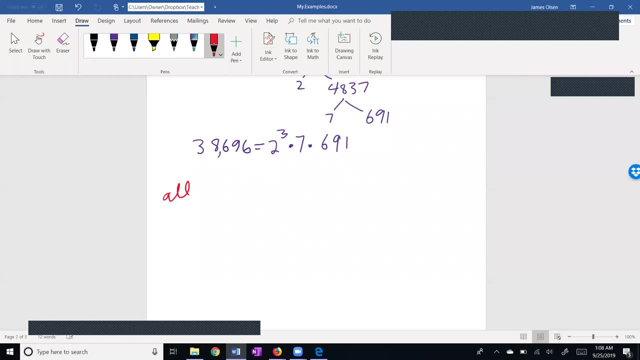 gives you one of the prime factors. So in this size, let's put together our form And all of the factors that construct the formula, as one should be the one that forms the formula times 391.. These are the three prime factors in this particular case, That there. 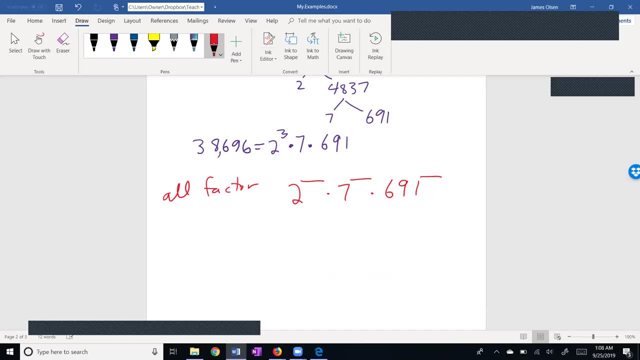 won't always be three prime factors, but this one happens to have three, be three prime factors, But this one happens to have three. Okay, The exponent on six, nine, ten to the power of zero. this is the reading, our form, with the. 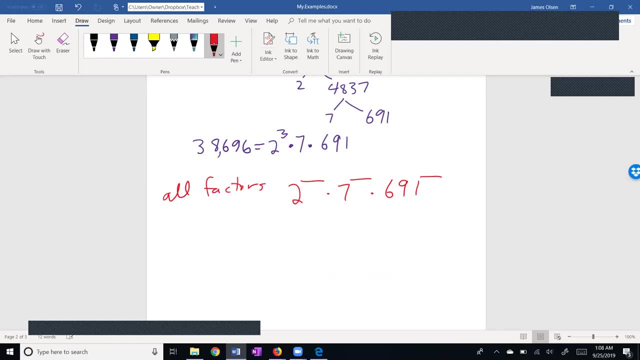 So 691 in all of our factors is either going to be a 0 or a 1.. The exponent that goes on 7 is 0 or 1.. The exponent that goes on 2, I've got some possibilities here- I could have 0.. 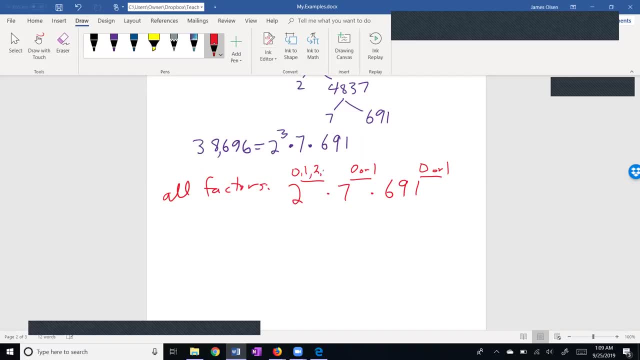 I could have 2 to the first, I could have 2 to the second, Or I could have 2 to the third. So my choices on my exponents. I've got 4 choices for the exponent on 2,, 2 choices for the exponent on 7, and 2 choices for the exponent on 691. 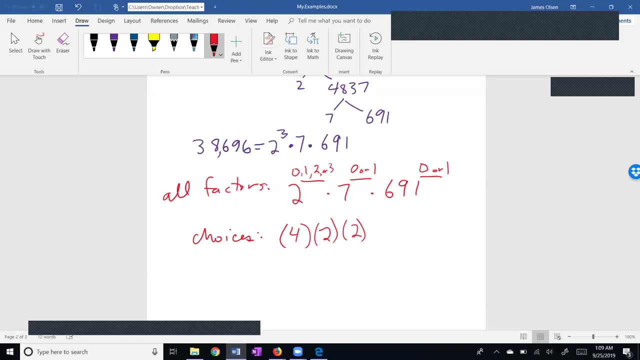 The fundamental counting principle in mathematics says that if we have choices, we multiply. there are 16 factors, So if we have choices, we multiply, we get a total of 38,696.. I like to do the example of t-shirts and gym shorts. 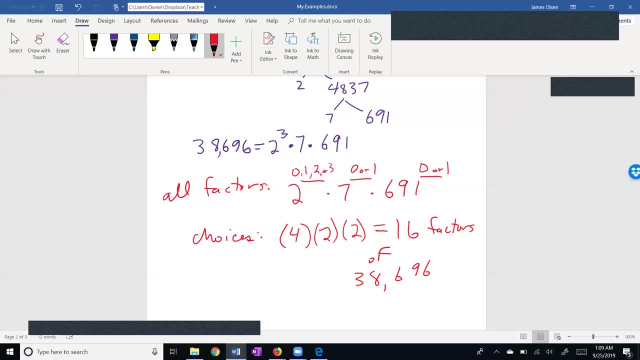 If I've got 3 pair of t-shirts or 3 t-shirts and 4 pairs of gym shorts- and I don't care what goes with what- 3 t-shirts and 4 pair of gym shorts- I have 12 outfits. 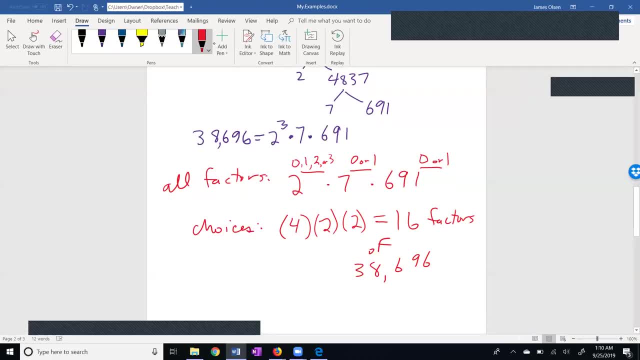 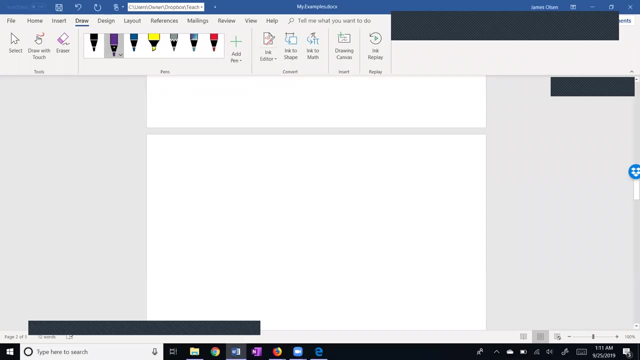 The fundamental counting principle says that you multiply. Now let's generalize this. Okay, so let's say our number n is, in its prime factorization form: p1 to the power of e1, times p2 to the power of e2.. Times p3 to the power of e3, through pn or pk, we'll say times, I'm sorry. pk raised to the power of ek. 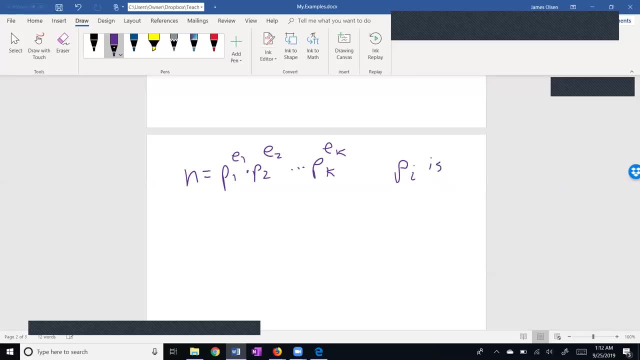 So p sub i is prime And the e's are the exponents. The number of factors of n. Number Of factors of n Equals E1 plus 1.. Times e2 plus 1.. Times e3 plus 1.. 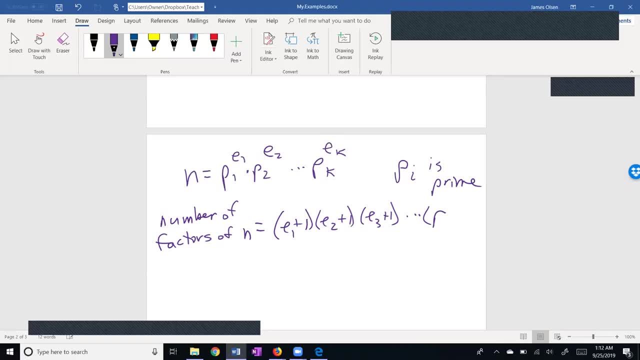 Times times, times Through Ek plus 1.. And the reason we have the plus 1 is because I can have an exponent of 0. In fact, all the exponents could be 0. If all the exponents are 0, that gives me the factor of 1.. 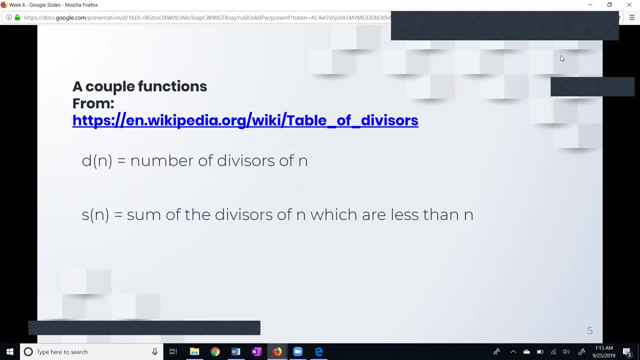 Now I'd like to look at a little bit of notation here. Remember, the number of divisors is what we just calculated. We're going to use dn for that. d of n is the number of divisors of n. So the number of divisors of a prime number is 2.. 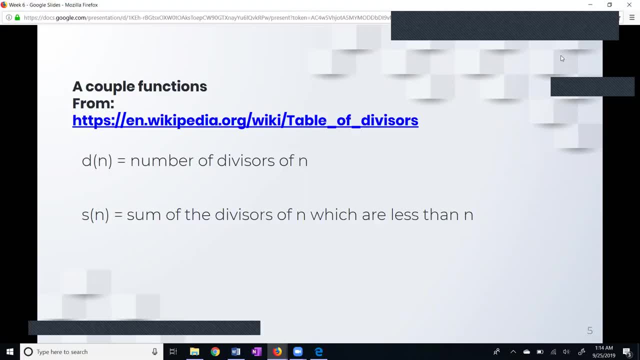 d of 7 is 2.. d of 11 is 2.. The number of divisors of 4 is 3.. We're also going to have another little function here, called the sum of the divisors of n which are less than n. 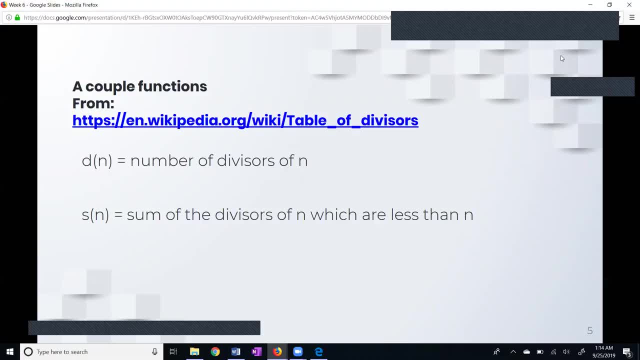 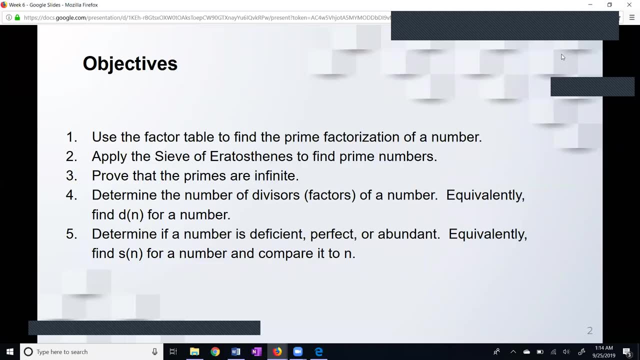 So our next objective, our final objective, in fact, determine if a number is deficient, perfect or abundant. Equivalently, find s of n For a number and compare it to n. Let's look at the perfect numbers. 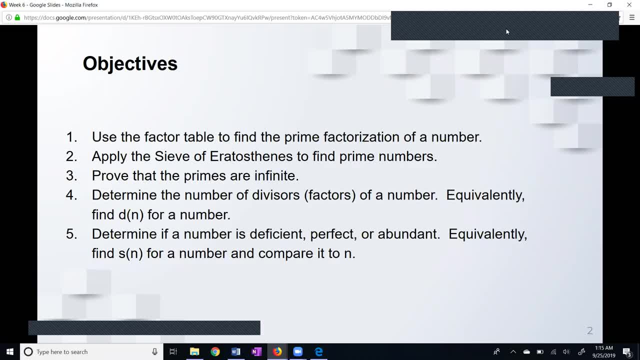 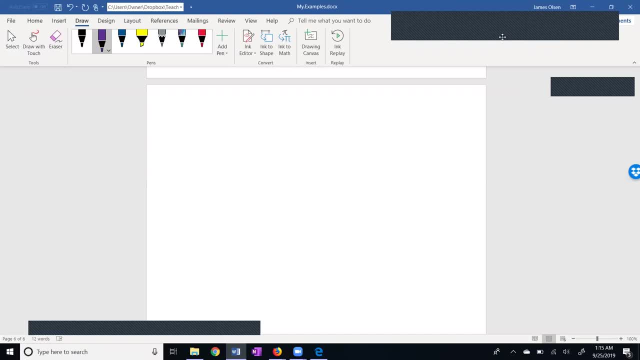 The first perfect number is 28.. I'm sorry, did I say the first perfect number is 28?? The first perfect example that I'm going to do is 28.. The first perfect number is actually a 6.. Let's show the 28.. 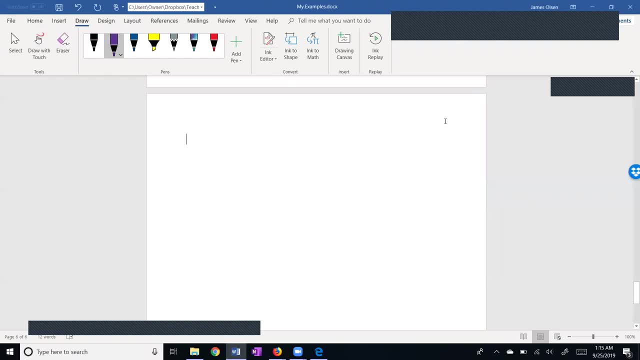 28 is a perfect number. So the first thing we do is we list the factors of 28.. 1 and 28.. 2 and 14.. 3 does not go in 4 and 7. And then we take the sum of the numbers. 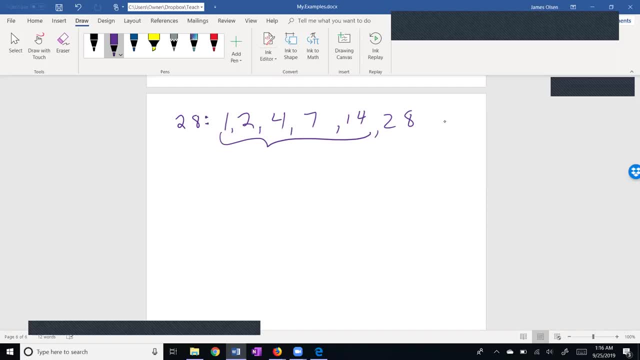 Let's see. Let's see, Not including 28.. 1 plus 2 plus 4 plus 7 plus 14 equals 28, exactly. Exclamation point 28 is perfect. Now this is a pretty easy process. Once again, nice little thing. 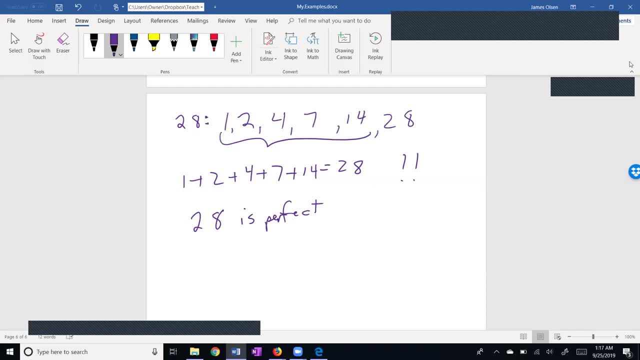 Nice little thing for middle school students to do: Determine if. well, let me give you the other terms. If you add up the divisors less than the number and you get something smaller than the number, the number is called deficient. A poor thing. 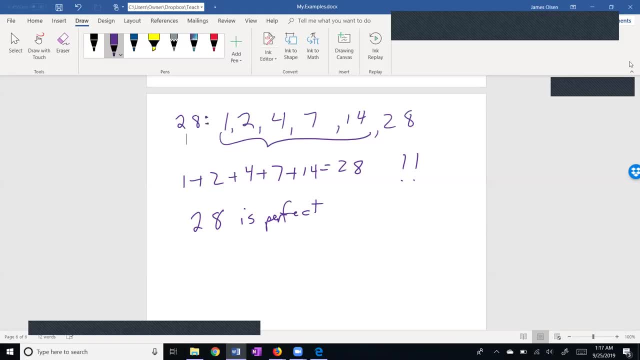 It's deficient. If you add up the divisors and you get a sum that's greater than the number, it is abundant, So let's do 27.. The divisors of 27 are 1 and 27,, 3 and 9.. 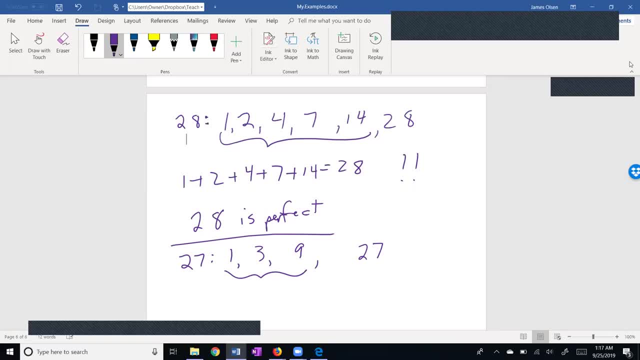 So if we add up 1,, 3, and 9,, S of 27 is 13.. I forgot to put my notation up here. S of 28 equals 28.. S of 27 is 13.. Since 13 is less than 27,, this means 27 is deficient. 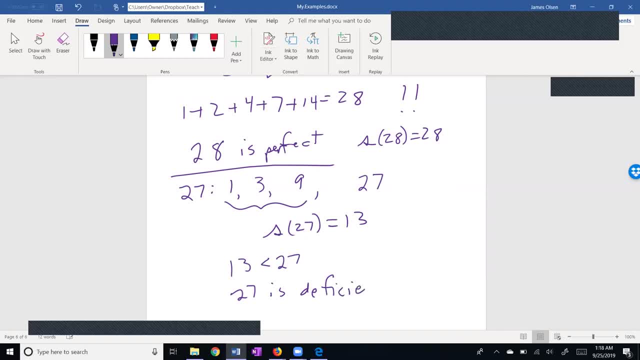 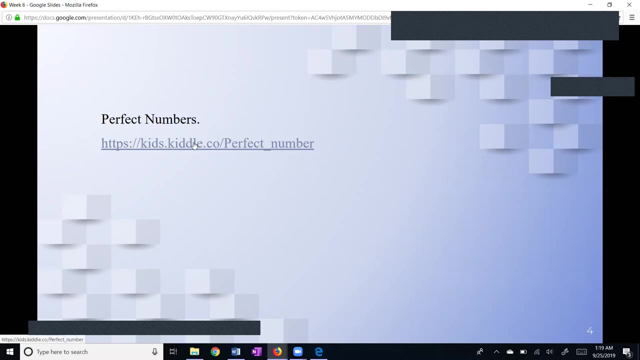 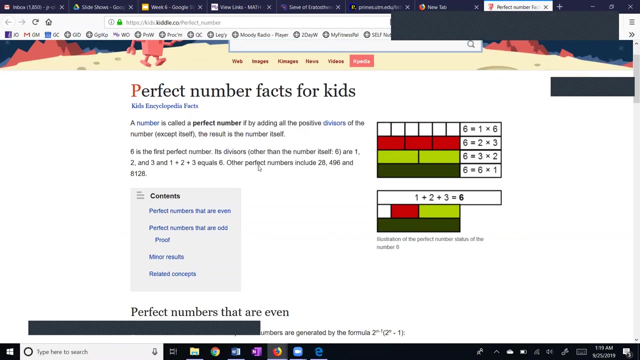 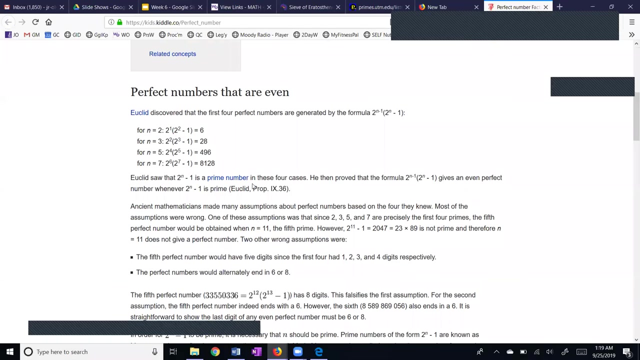 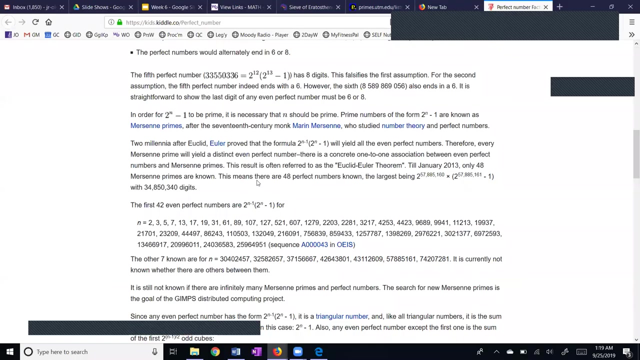 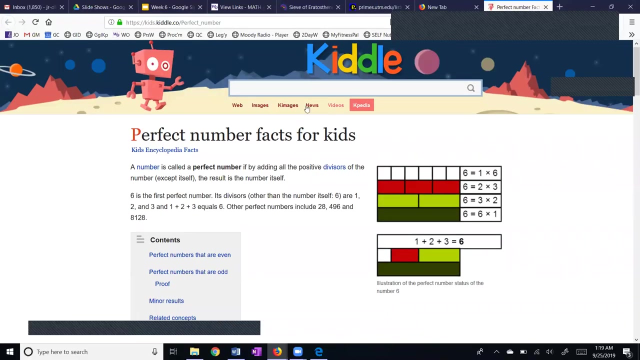 By the way, I found a nice website here, kidskindleco slash perfect number, And this is designed for kids and it talks about perfect numbers and gives some other interesting facts. It talks about perfect numbers and Mersenne primes. So what I'd like to look at next is a Wikipedia page. 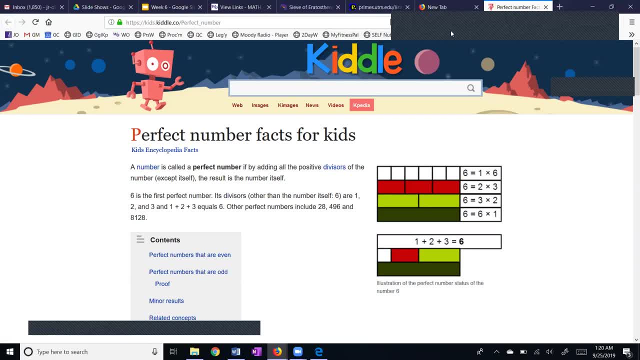 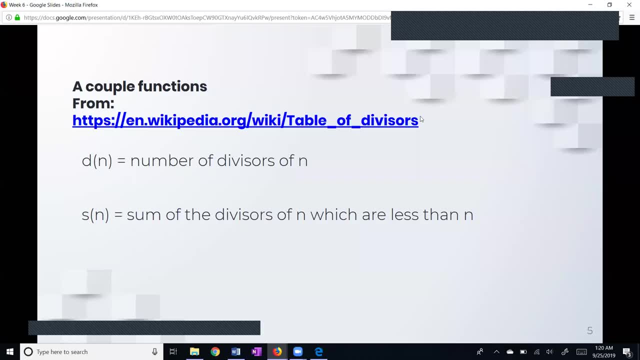 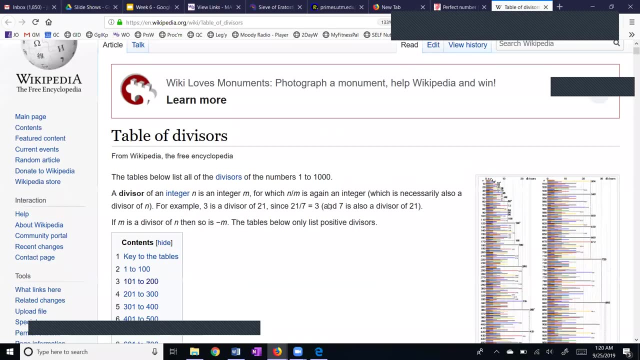 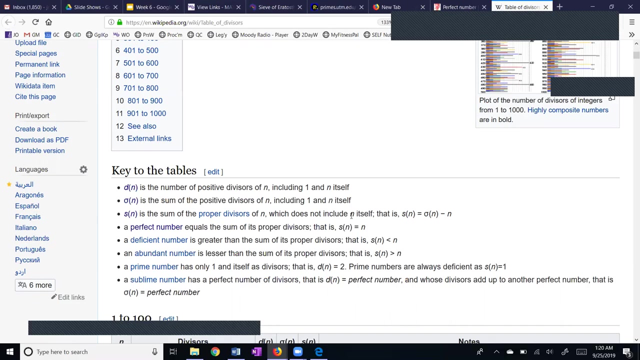 And I believe we have this. I've got the address for it here. Hang on a second. Yes, it's the Table of Divisors Wikipedia page, And this is nice. Here is the sum of the divisors, not including N itself. 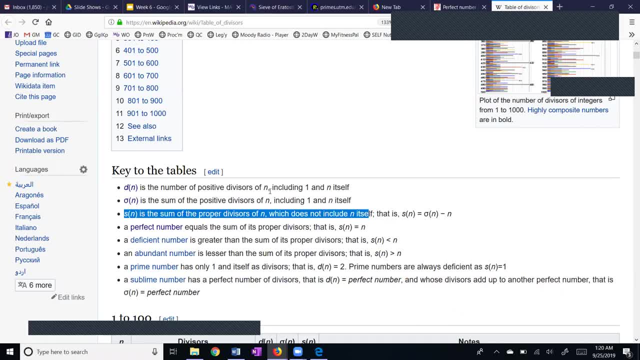 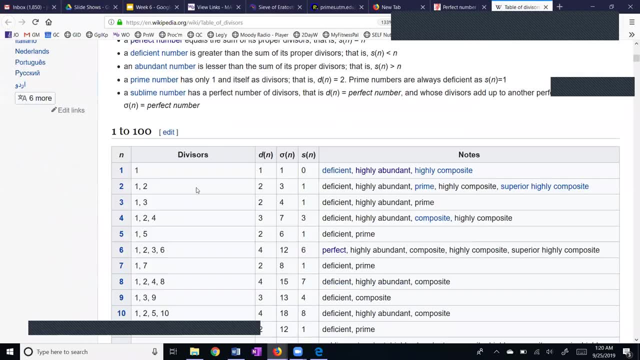 I'm using the same definition that Wikipedia is using, And D of N is the number of divisors, The number of divisors. And here we are, Here, we are, Here we are. Here's D of N, Here's S of N. 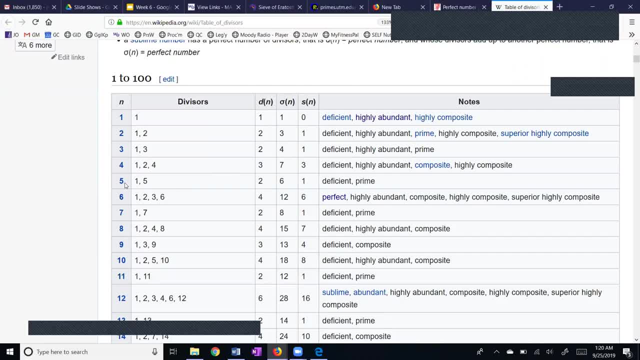 So let's take the number 5,, for example. D of N is the number of divisors, which is 2, because it's prime, And the sum of the divisors less than the number is 1.. It's woefully deficient. And it's prime. The number 8, D of N is 4.. It has 4 divisors And the sum of the divisors less than 8,, 1,, 2, and 4 is 7.. It is deficient. 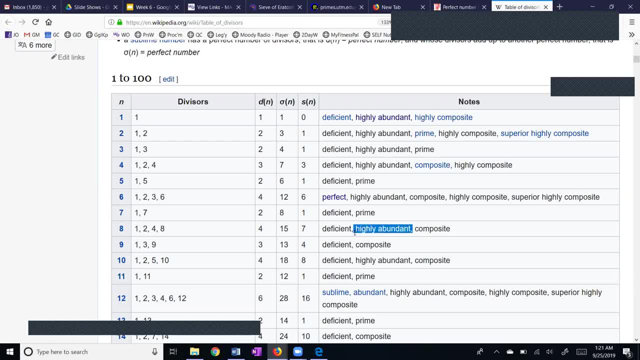 And it's composite. By the way, this term highly abundant. don't worry about that. It's kind of an odd term and not a common term. So don't worry about being highly abundant or not. So we have 6,, which is a perfect number. 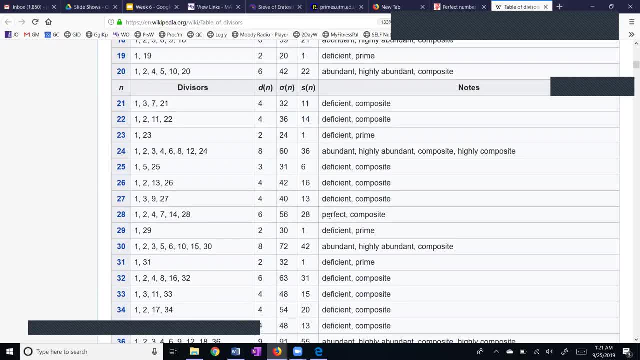 We have 28,, which is a perfect number. Here's 30.. Here's 30.. 30. 30 is kind of interesting. 30 is an abundant number. D of N. it has 8 divisors, And if we add up the divisors less than 30, we get 42. 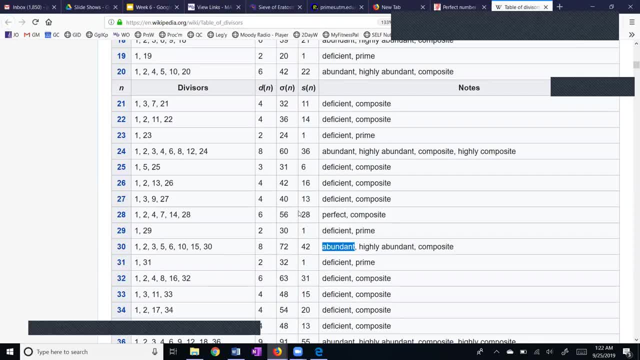 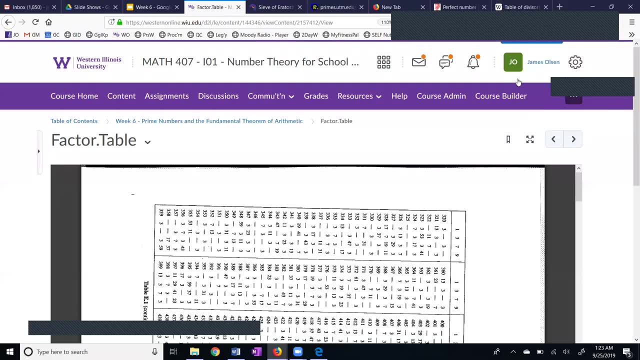 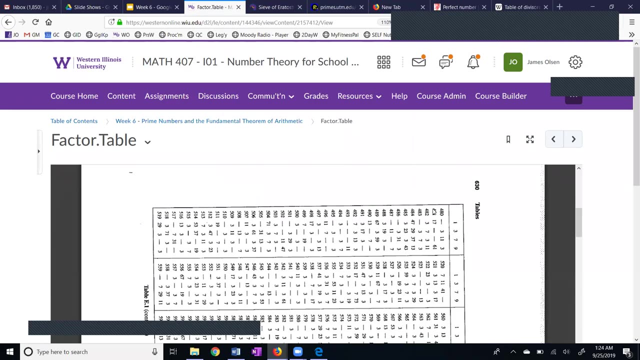 And 42 is larger than 30, which makes it abundant. Maybe what I'll end with is this factor. Let's look at the factor table. I was not able to find on the Internet. I searched for probably 25 minutes, So I'm going to offer 5 points of extra credit to any student that can find the factor table.